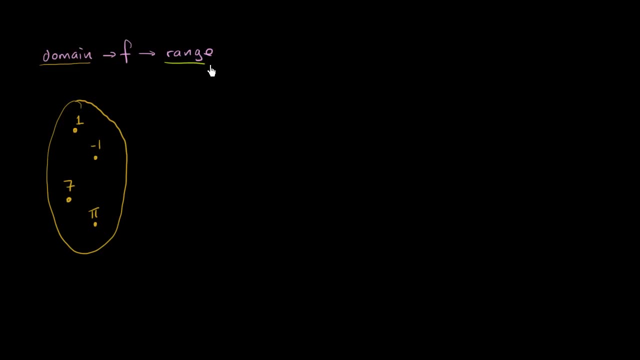 And let's say that f, and let's say that this right over here is the range, so this is right over here is the range. And so let's say that f of one, f of one, so if you input one into the function, 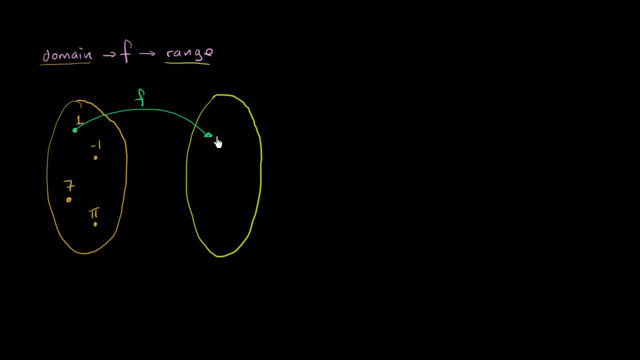 the function maps one to the number negative three. And let's say it maps the number negative 1, so f of negative 1 is equal to 7.. And let's say that f of 7 is equal to 10.. But let's say that f of pi is also equal to 10.. 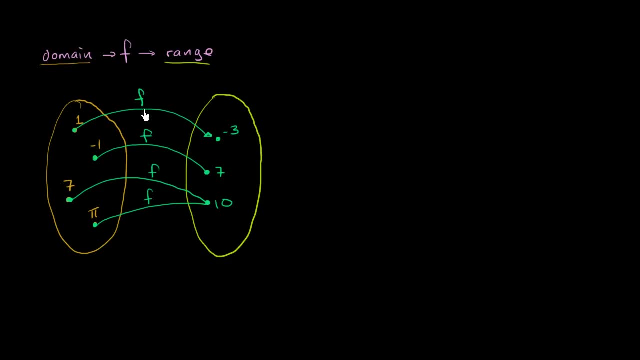 So this is the function mapping, And this is a legitimate function. Remember, in order to be a function for any input, it has to map it to a unique, it needs to map it to only one output. This wouldn't be a function if it did something like this. 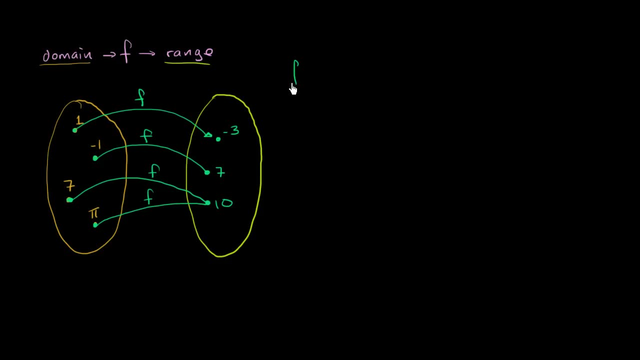 If you input pi, instead of saying you're going to get 10, instead of saying that f of pi is equal to 10,, this is clearly a function You're mapping from pi to 10.. For the input pi: you know you're. 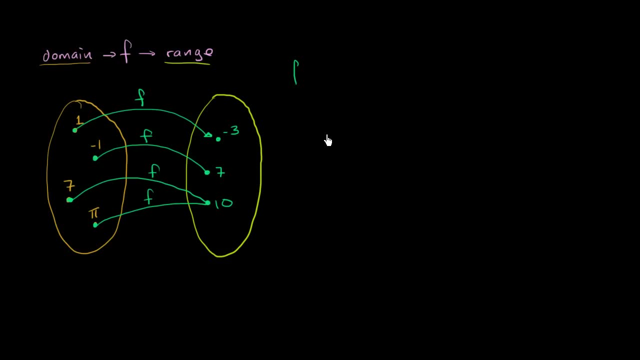 going to get the output 10.. But if you were doing some type of a relationship where you said, oh well, if you put in a pi, sometimes it's a 10, and sometimes it's an 11. Now this would not be a function. 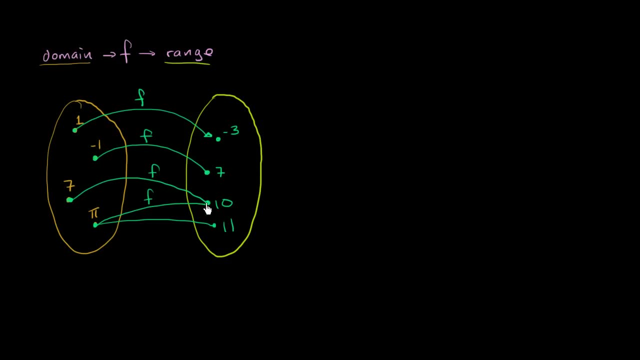 because you're mapping pi to two different values right over here, So that's not allowed. if you're thinking about a function For any input, you have to map it to only one output. Now you could have two inputs that map to the same output. 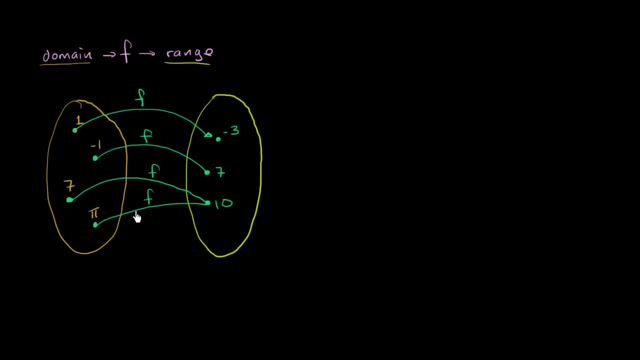 because this is predictable. You know that f of 7 is 10, and you know that f of pi is 10.. But what I want to do is now think about when is it not invertible? We've already seen that the inverse of a function 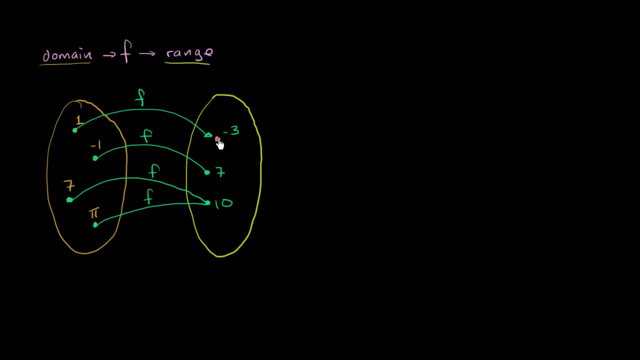 should map between an element of its range and the corresponding element And the domain. So the inverse of f should map negative 3 to 1.. So f inverse. So because f of 1 was equal to negative 3,, f inverse of negative 3, and the inverse function. 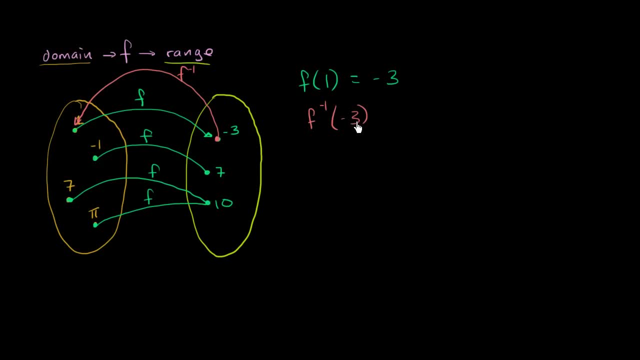 is also a function, so it has to have the same properties of a function. It should map to only one thing. So f? inverse of negative 3 is going to be equal to 1.. f inverse of 7 is going to be equal to negative 1.. 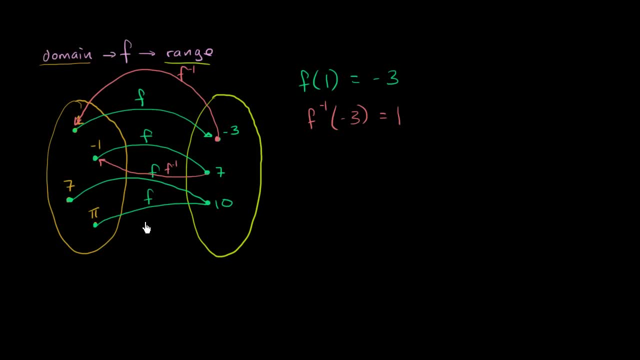 f inverse. this is f inverse right over here. But now we have something strange happening If we think about so. let me write this down: f inverse of 7 is equal to negative 1.. That makes sense, because we already knew that f of negative 1 is equal to 7.. 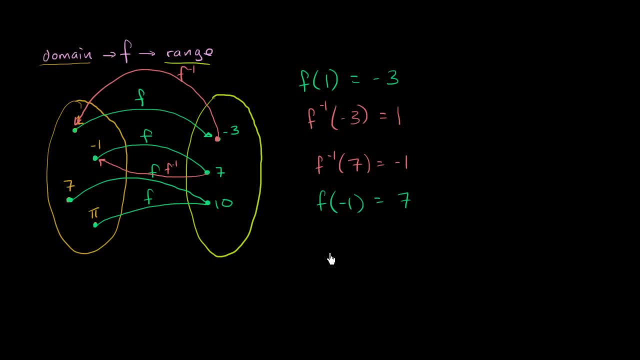 But now something interesting happens over here. What would f? f inverse of 10 be? Well, f inverse of 10, if I'm trying to map it, 10,. there's two elements of the domain that, when I applied the function, got us to 10 in the range. 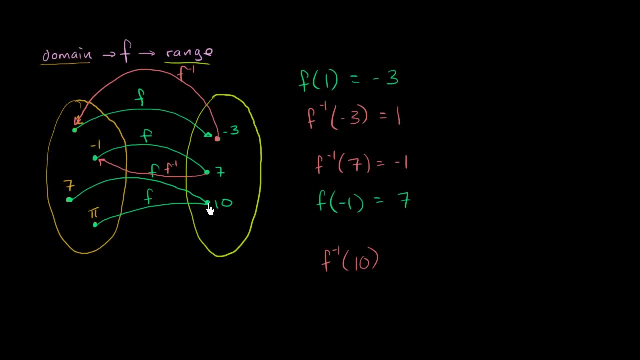 So if you're trying to see whether f is invertible, then the inverse function should map this element to only one element of the domain, But it's mapping it to two elements of the domain. So is this equal to 7? Or is this equal to pi? 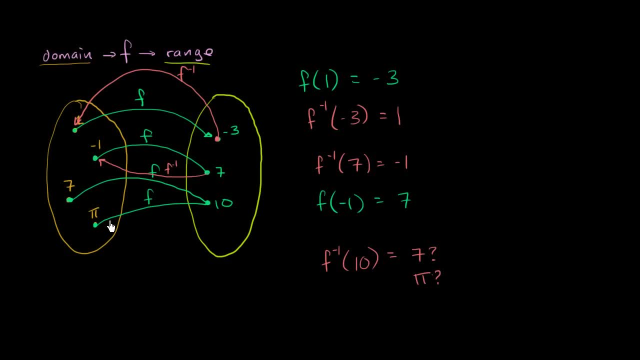 Or is this equal to pi? Or is this equal to pi? And because the inverse mapping can't be done, where you only map it with a unique thing, this function is not invertible. This is not invertible: The inverse mapping from the range to the domain. 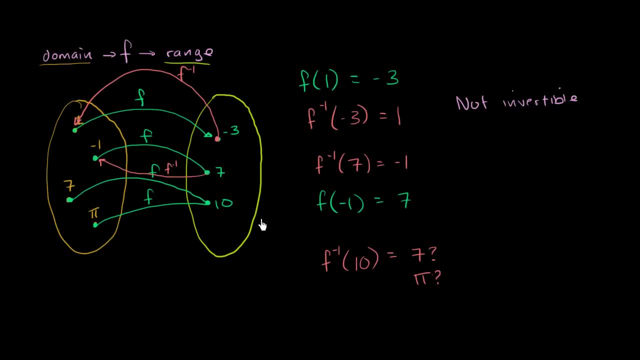 the inverse relationship is not a function. It can't take an element in our range and map it to a unique element to the domain For 10, we don't know, Does that map to pi Or does that map to 7??